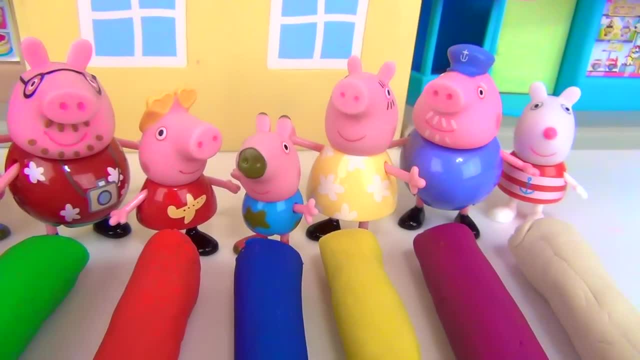 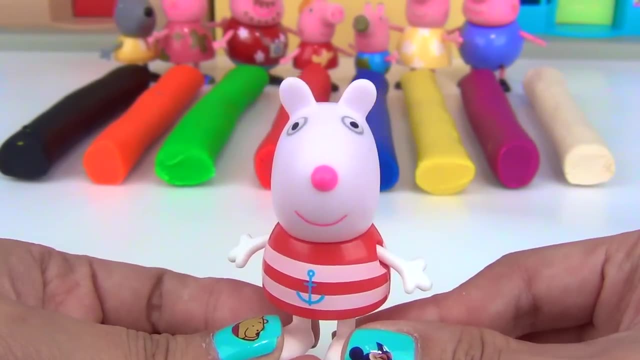 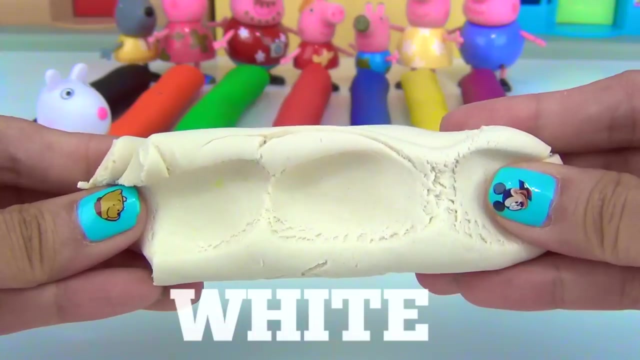 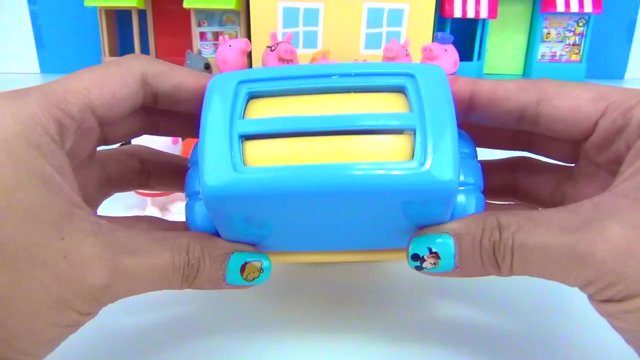 for Toys Unlimited, and today we are going to have fun with Peppa Pig, her family and some of her friends. We are going to start with Susie Ship. Here we have white Play-Doh. White Susie, would you like to have some toasts? That would be great. Here we have. 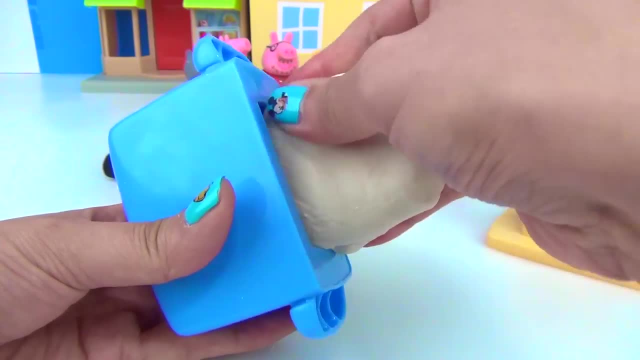 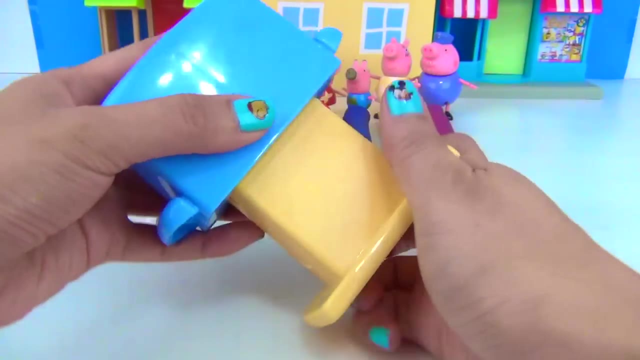 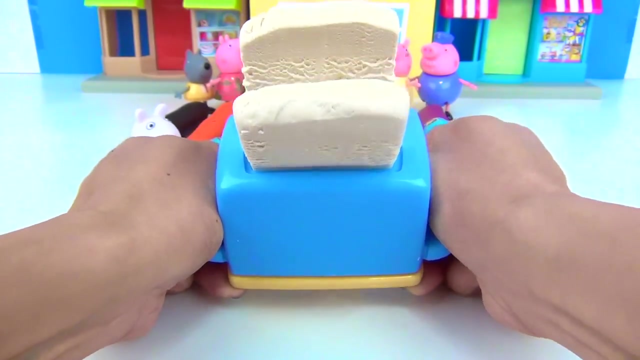 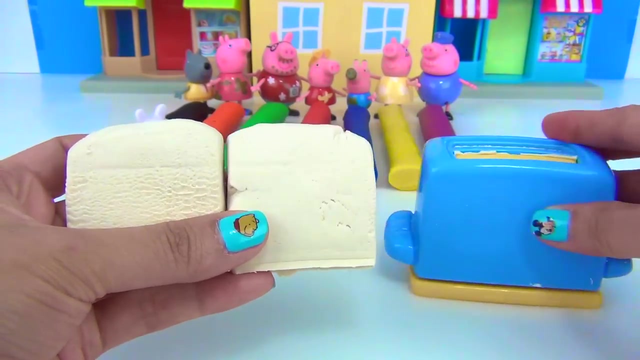 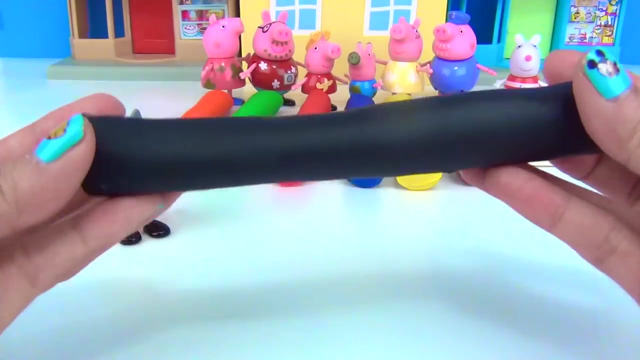 our toaster and all we have to do is put our Play-Doh in there, Just like that, And we push it in. Toasts are ready. Yay, the toaster works great. Pedro Pony is up next. He has black Play-Doh- Black. 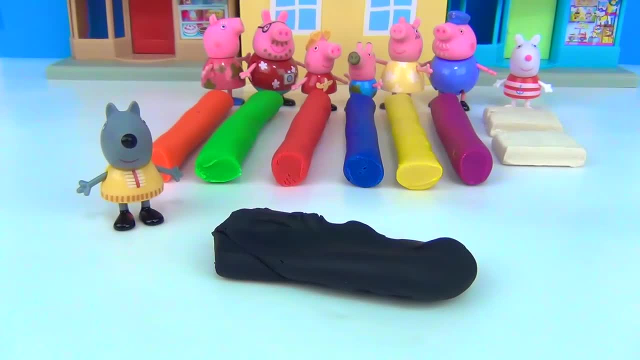 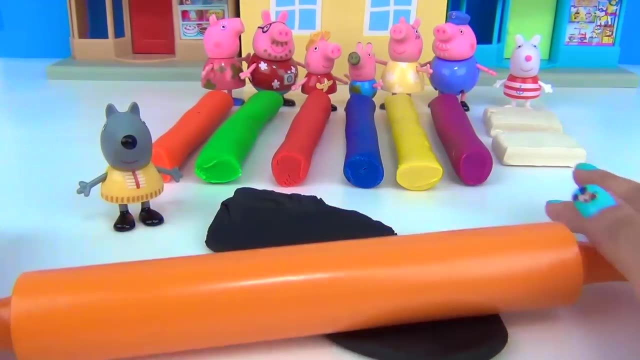 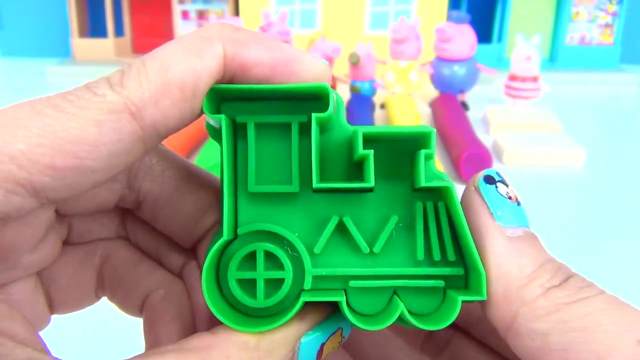 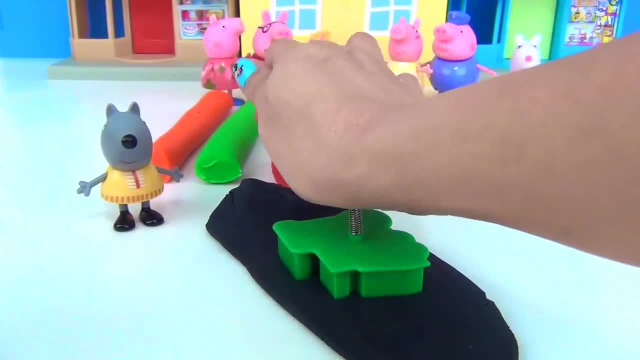 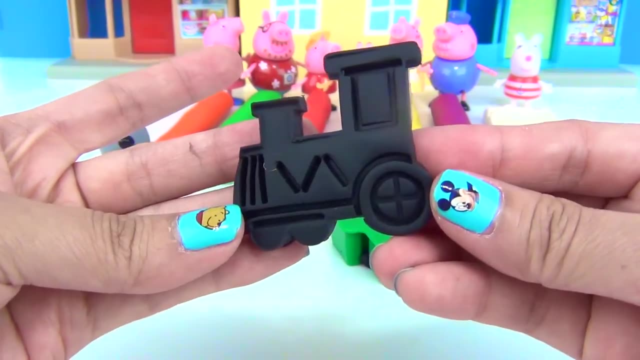 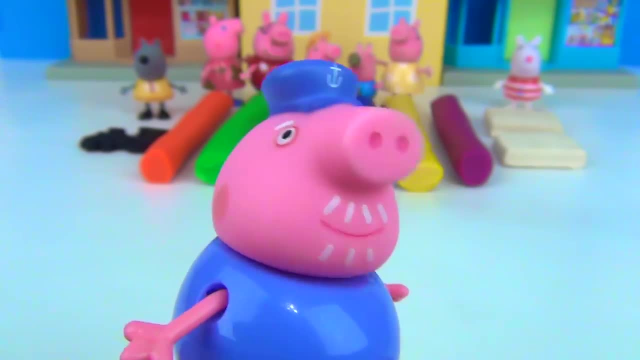 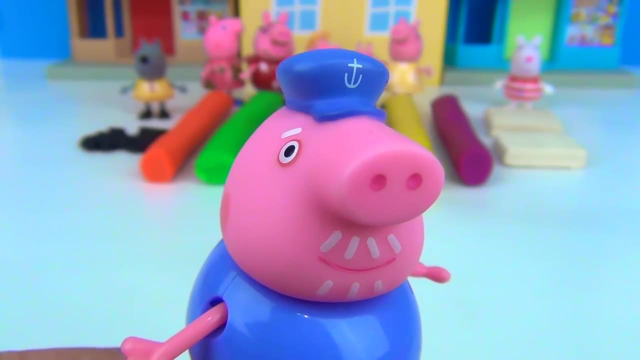 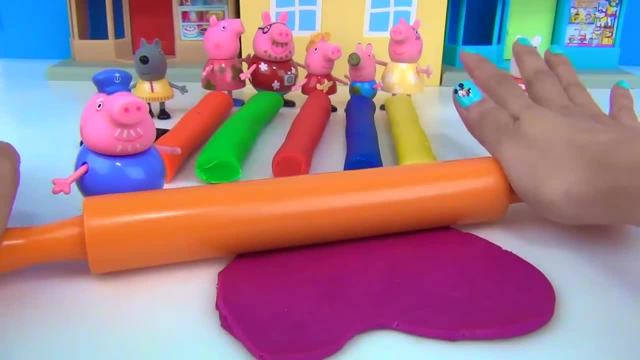 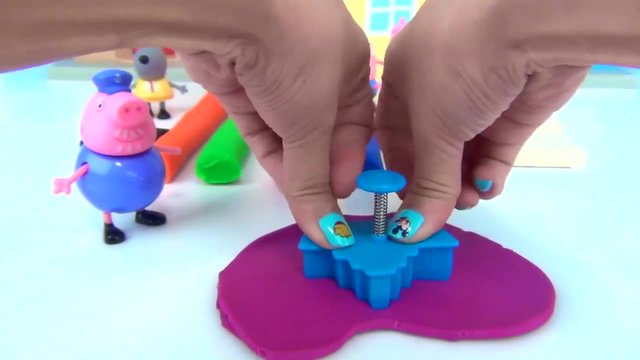 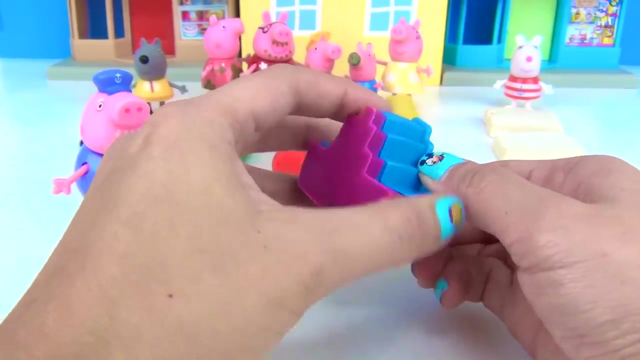 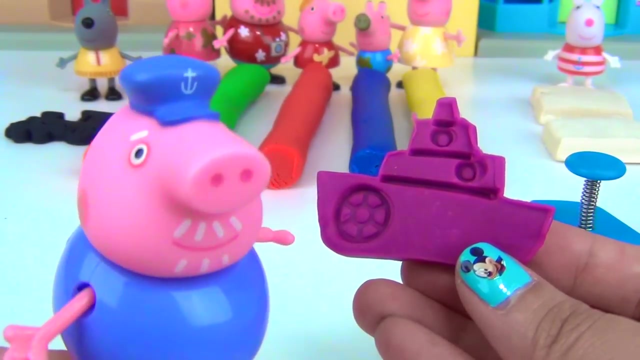 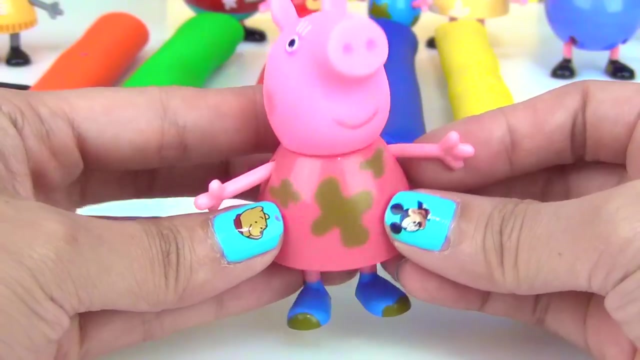 Submarine coming right up. Here you go, Grandpa Pig, Your very own purple submarine, Thank you. Up next we have Grandma Pig. Uh oh, looks like Grandma Pig has been playing in the muddy puddles. She has mud splatters. 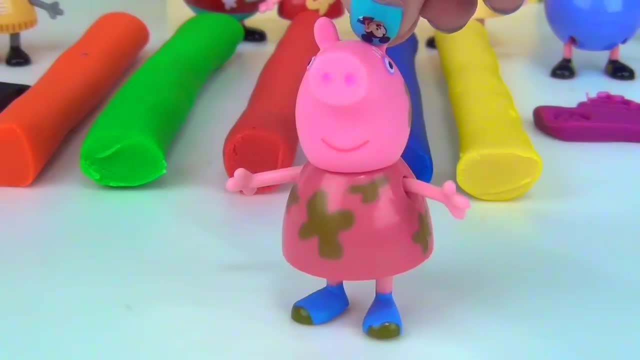 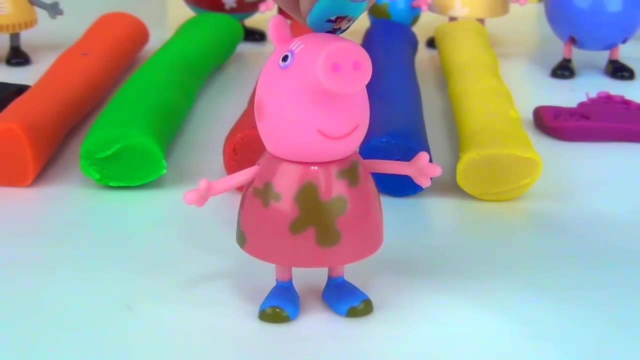 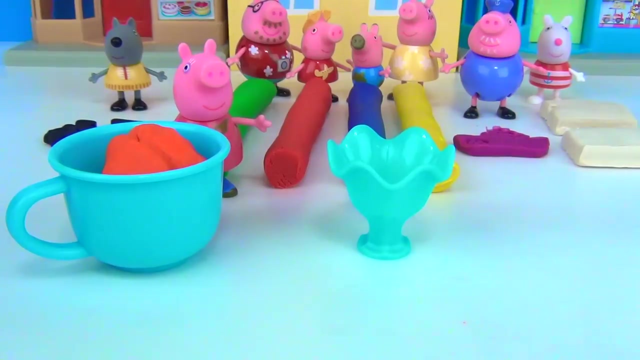 all over her. That's right, I love muddy puddles, but now I'm hungry. How about some scoops of orange ice cream To make an ice cream? let's go ahead and put our Play-Doh inside our container. Here is our ice cream cup, and let's get our scooper. 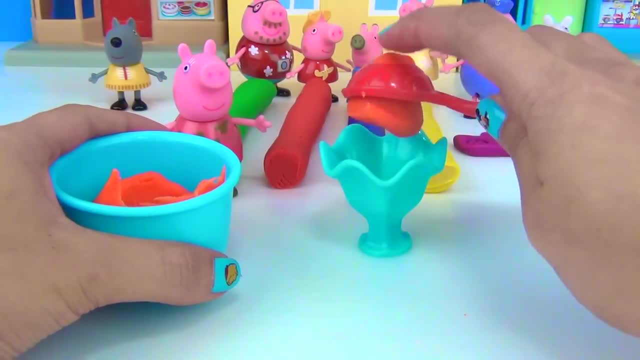 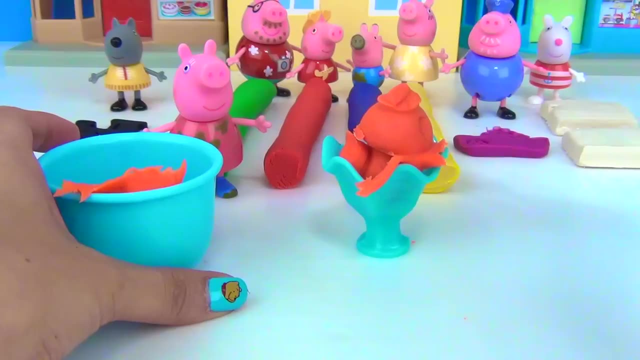 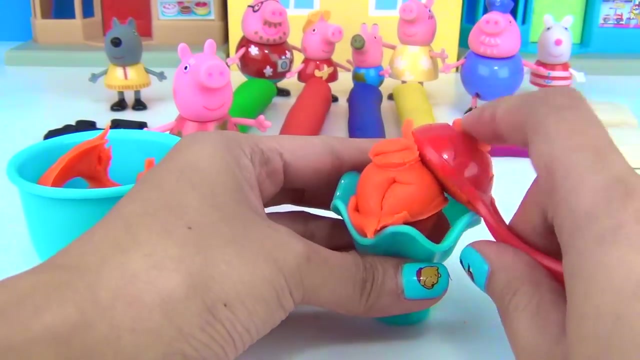 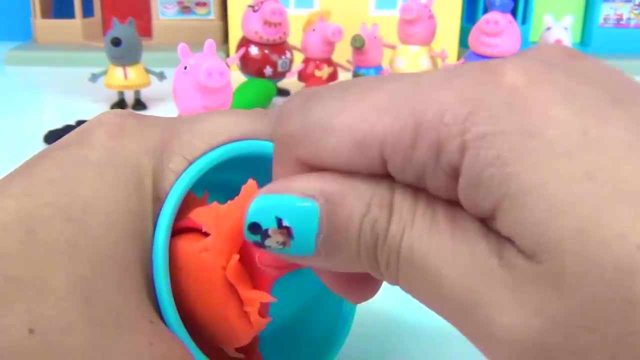 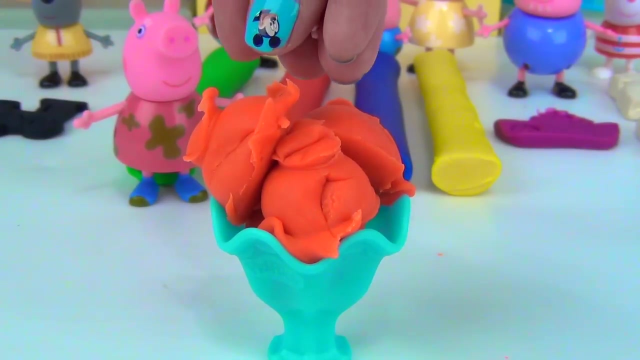 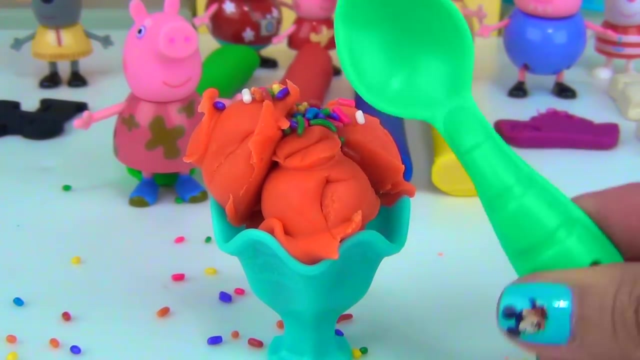 Cool, Cool, Cool. First scoop of ice cream, second scoop, third one- I think we can do one more- and four. Hey, how about some sprinkles a little bit more? and of course our spoon. Oh dear, it sure looks delicious. 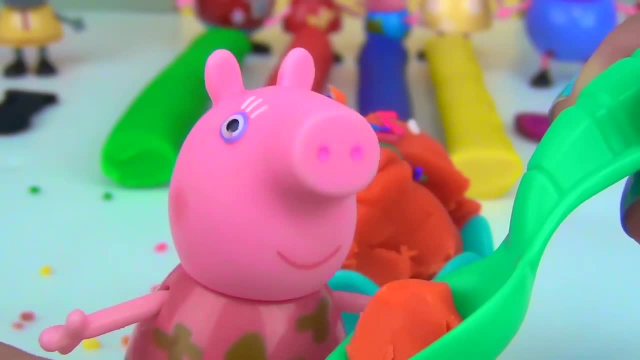 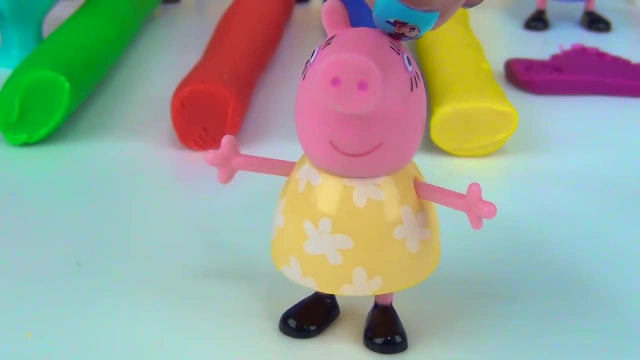 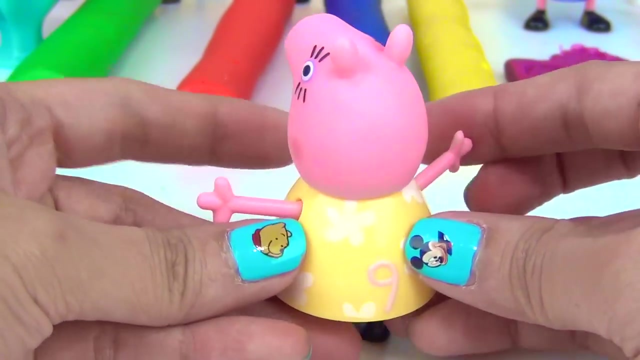 Let's give it a try. Grandma Pig. Yes, it is, Whoa. check it out, it's Mommy Pig. Ooh, Mommy Pig, I like your dress. It's yellow with some flowers. Mommy Pig has yellow Play-Doh. 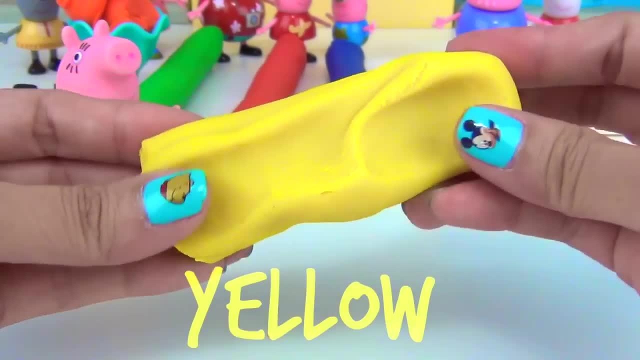 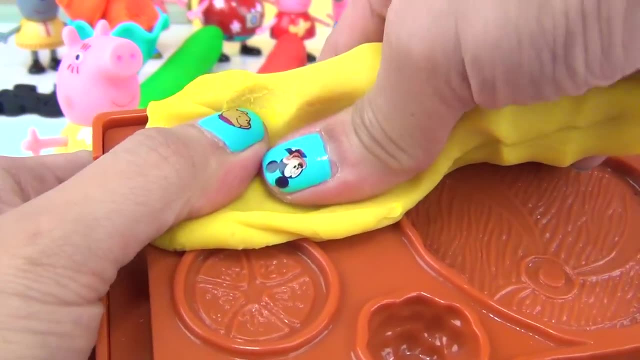 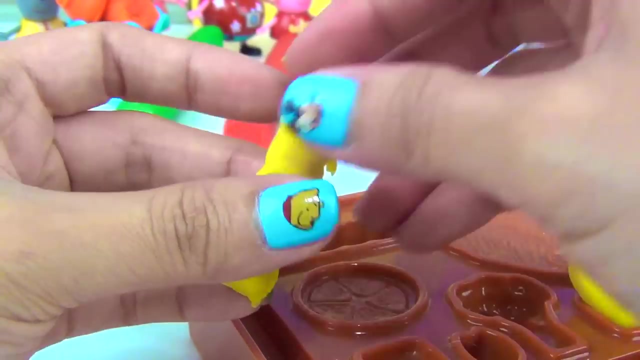 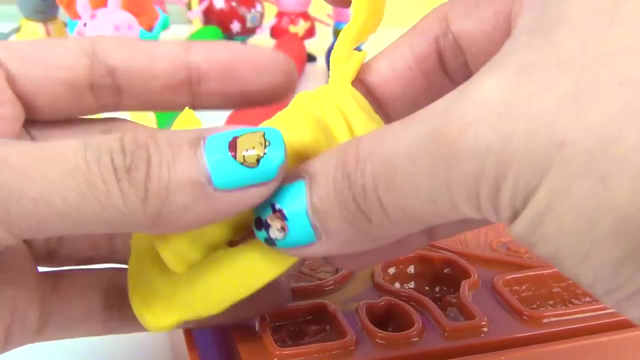 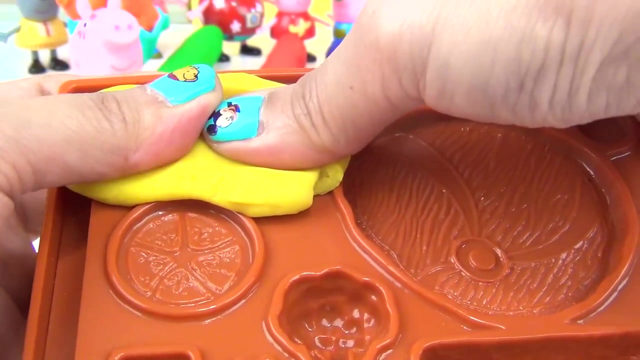 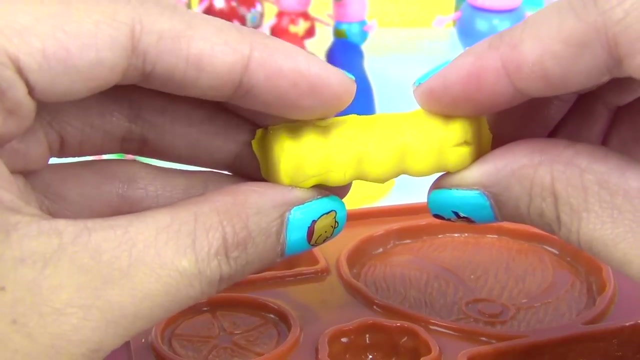 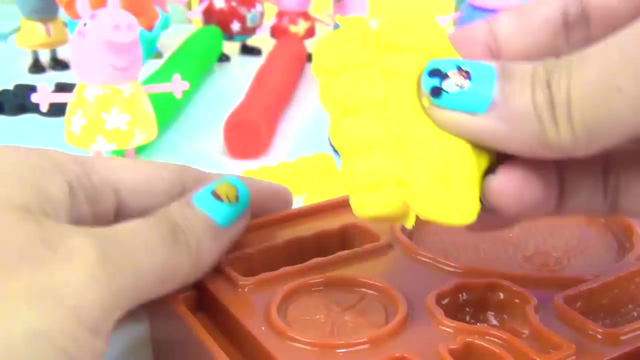 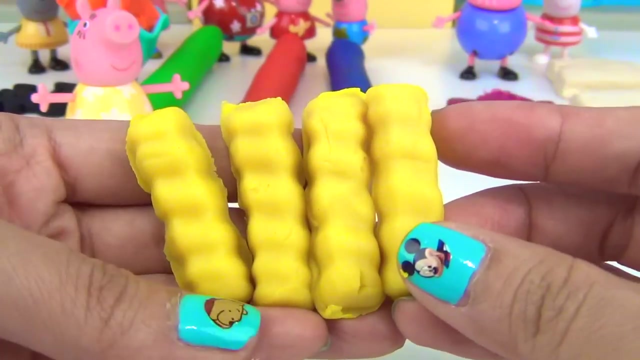 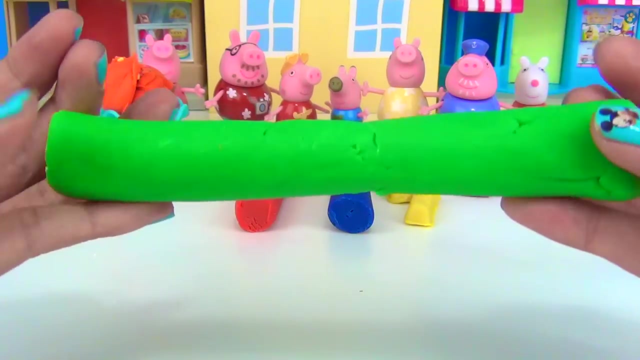 Oops, sorry yellow. And for her we should give her some french fries. One, Two, Three, Four. One, Two, Three, Four, Four french fries for Mommy Pig. Our next Play-Doh is color green. 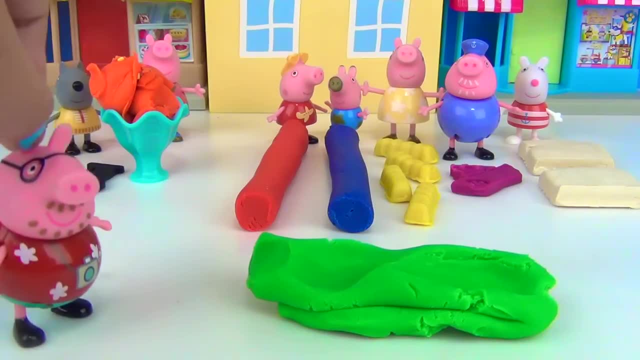 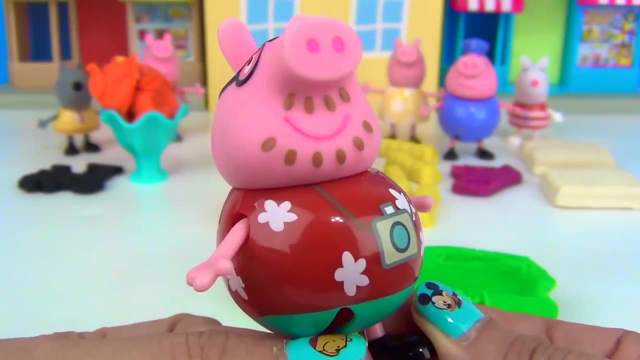 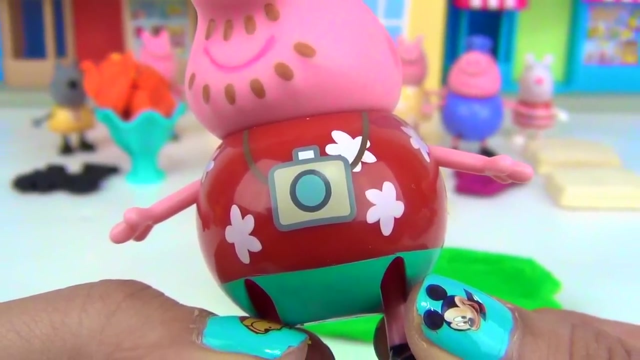 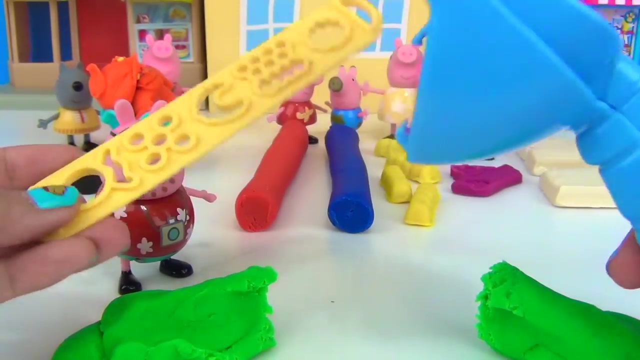 Green And it is Daddy Pig's Play-Doh. Daddy Pig is wearing a red dress and he also has a camera. Say, cheese, Cheese, Cheese, Cheese, Cheese, Cheese, Cheese. Okay, Daddy Pig, I think I want to make you some green beans. 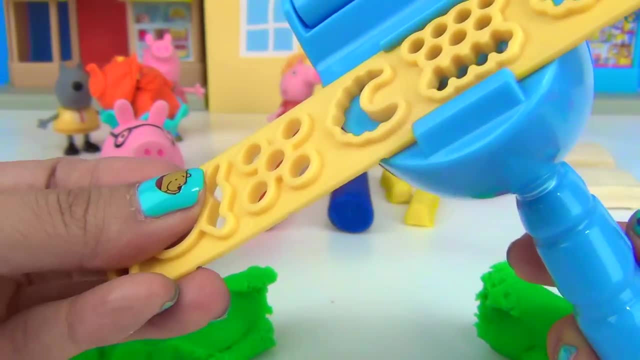 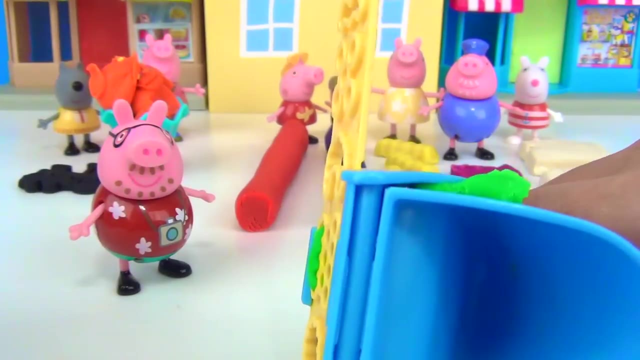 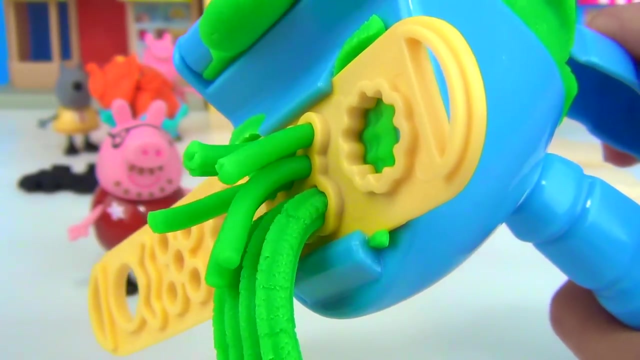 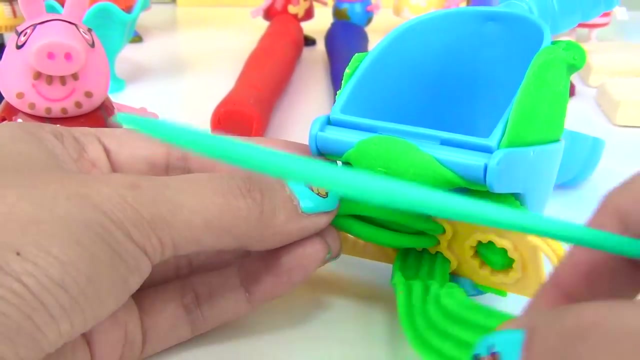 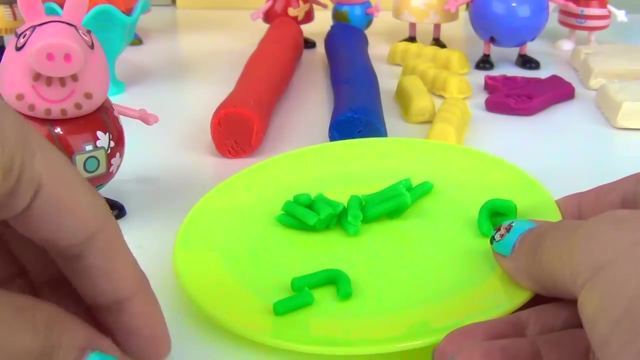 Here's what we're gonna need. Let's put that right here. Put our Play-Doh in the extruder and then we push it in. There's our green beans. Thank you, Thank you. We don't need that. Green beans on a green plate. 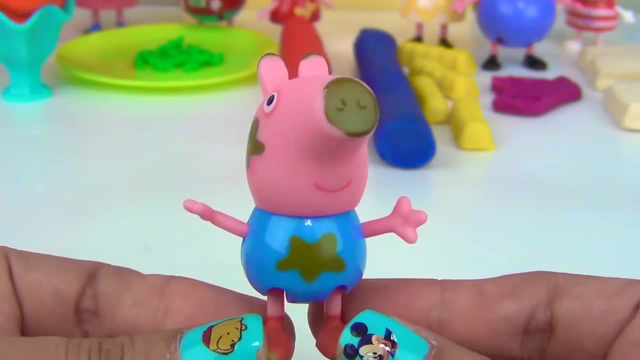 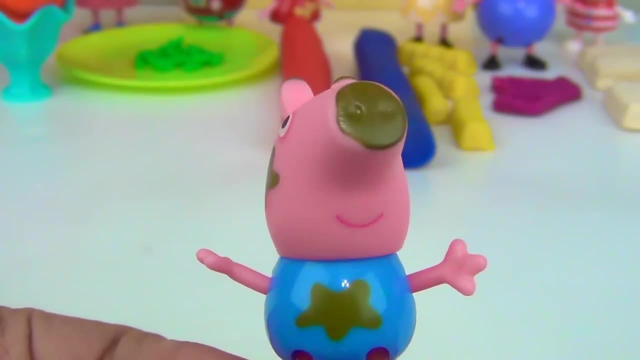 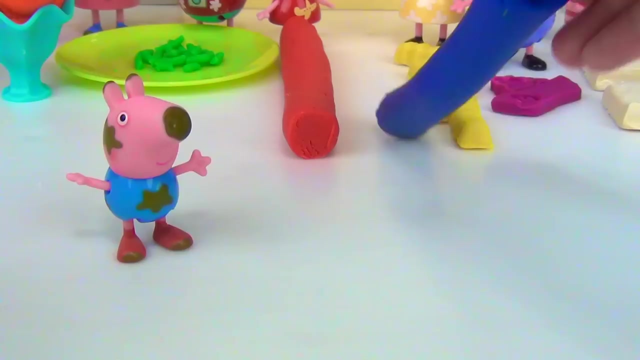 Yay, it's George Pig's turn. Uh-oh, George Pig has also been playing in the muddy puddles, Muddy puddles. Yep, that's right, he has mud splatters all over him. Okay, George, here is your play-doh. 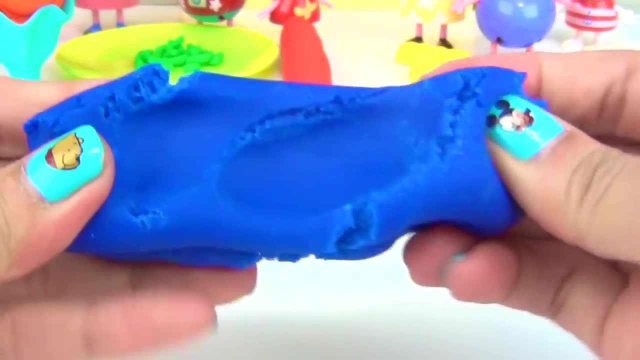 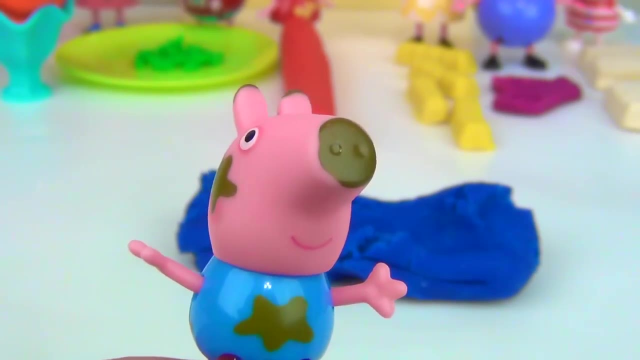 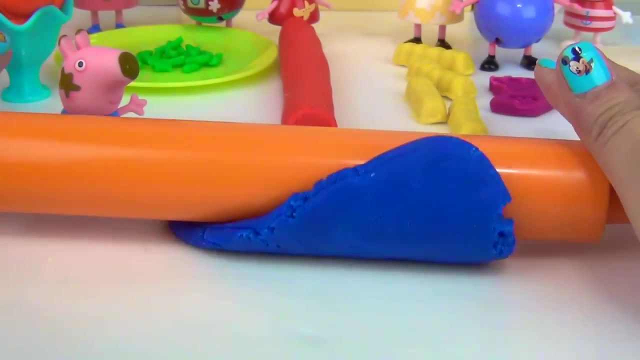 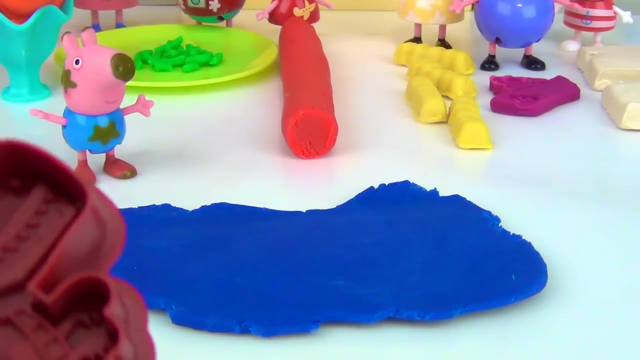 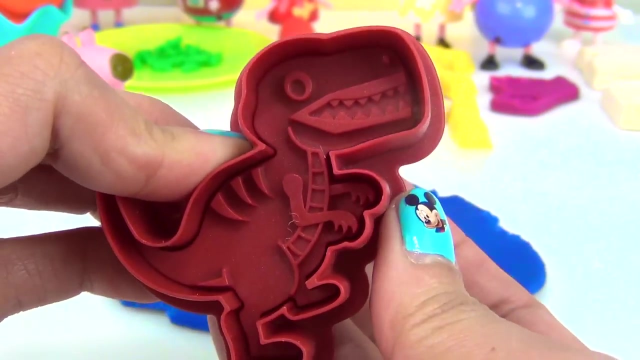 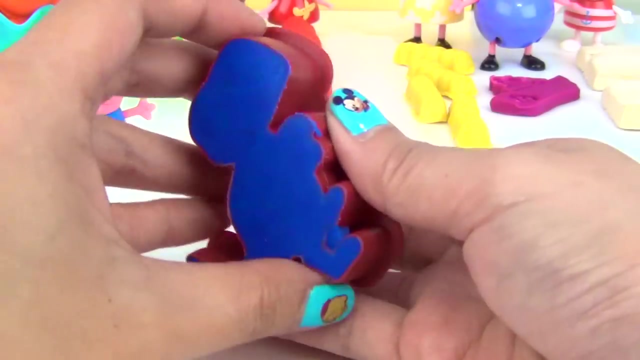 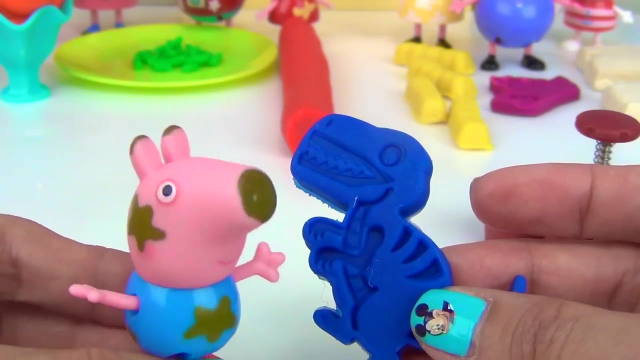 Color: blue Blue. What would you like me to make? I want a dinosaur Rawr. We can definitely do that. Let's just roll up the play-doh first. Here is our dinosaur Rawr. Oh, dinosaur rawr. 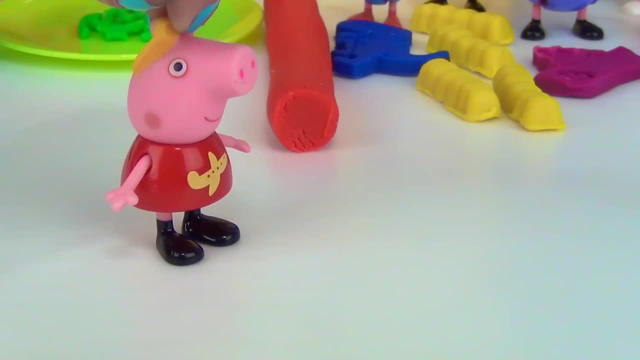 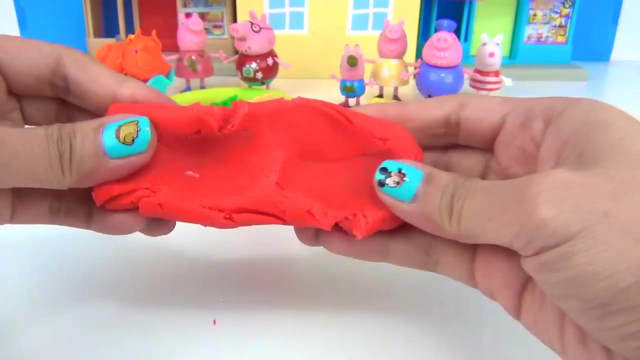 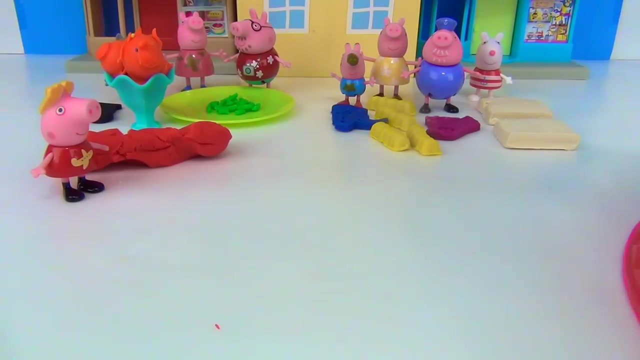 Rawr Rawr. Hi, I'm Peppa Pig and I have red Play-Doh, Red Play-Doh Red And I would like to have some red gumballs To make our gumballs. we are going to need our gumball maker.